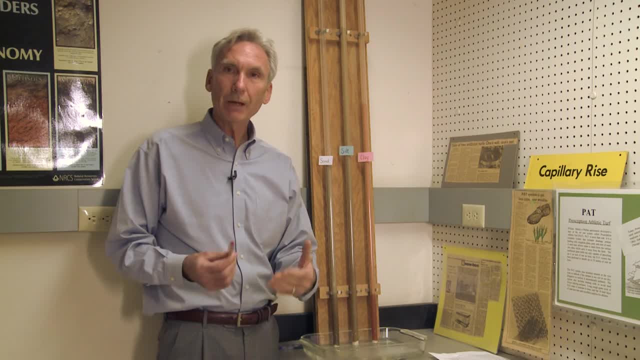 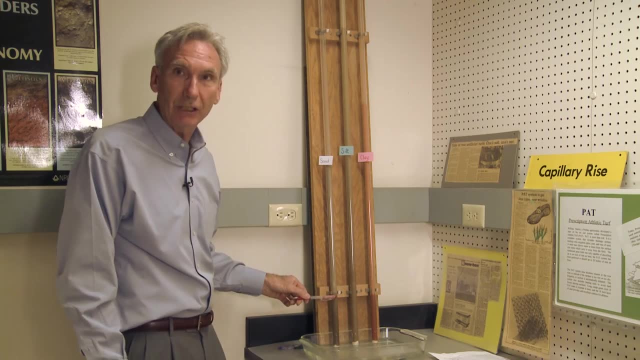 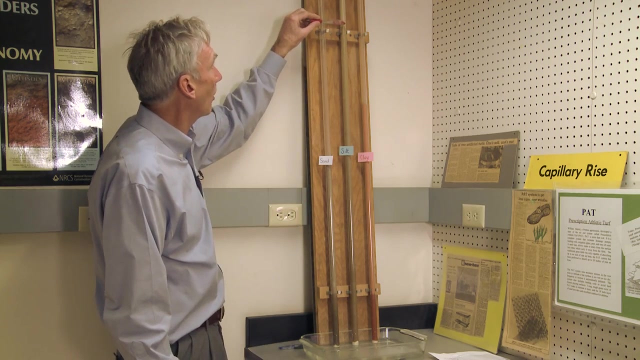 migrate up these three tubes And, as you would imagine, with the sand it doesn't migrate up nearly as far. it only goes up to about here. If we look at a silt, on the other hand, the silt migration goes all the way up to here. If you look at the 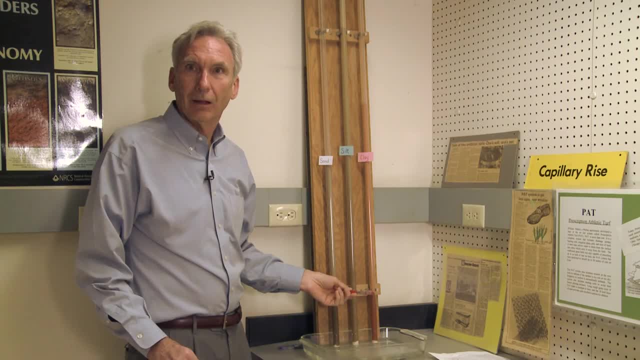 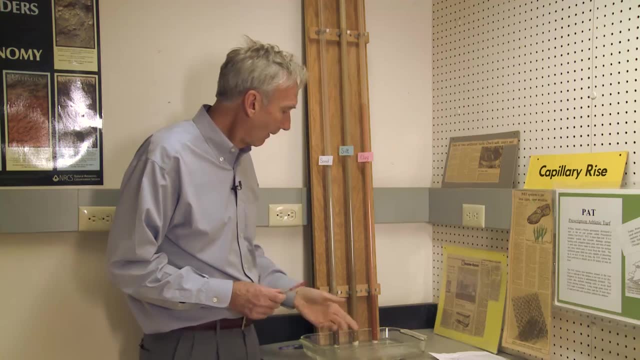 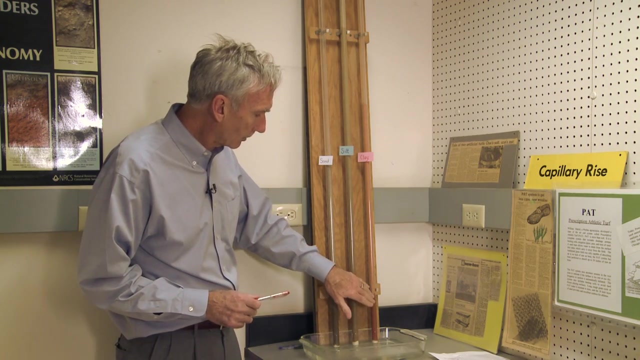 clay. it only goes about this high And you're probably asking: well, why is that? It has such small pores? you would think that it would migrate up very high. Essentially, what happens with the clay is that When the water is absorbed in this tube, here, those small pores in the clay swell shut. 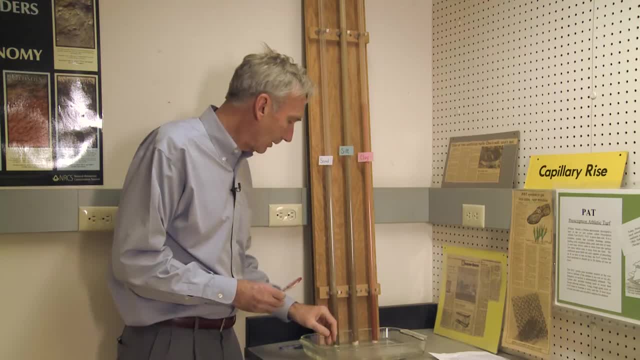 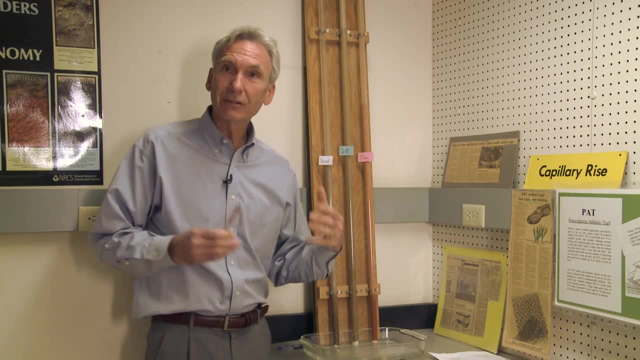 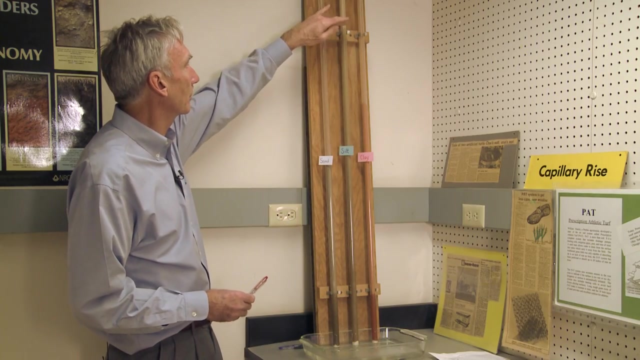 and it doesn't allow the water to migrate up very far. In the sand it has very large pores. it doesn't allow the water to migrate up very far. In the silt, it has a nice combination of large and small pores and what you find is that in a silt-textured type of soil you're 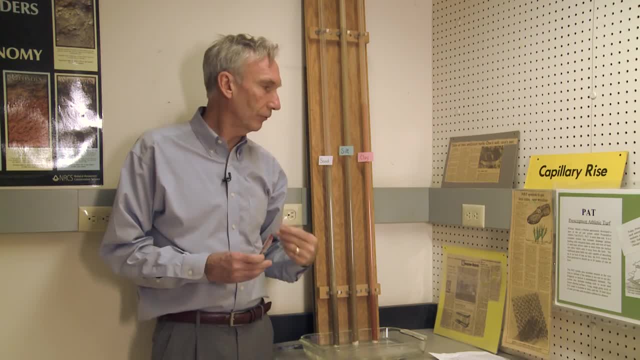 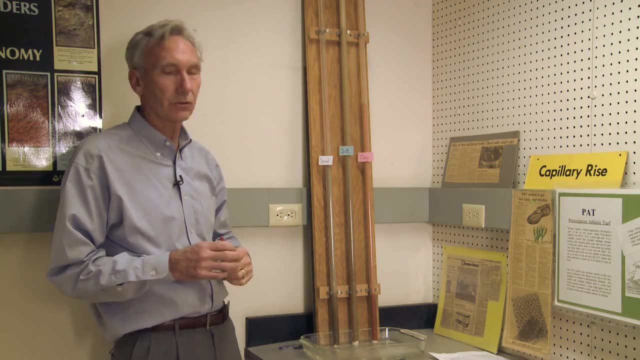 going to have the highest capillary rise of of any type of soil that you'll have. You'll see higher capillary rise in a silty-textured type of soil than you would in a sandy or a clay-textured type of soil. 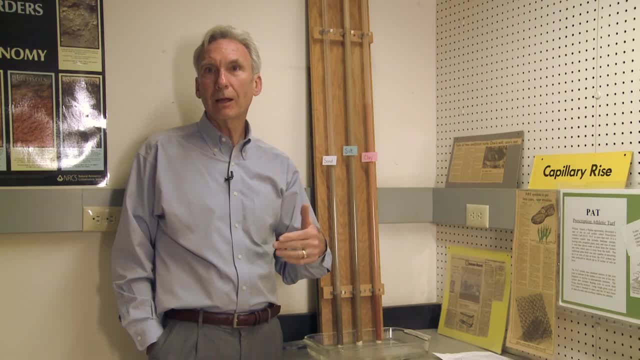 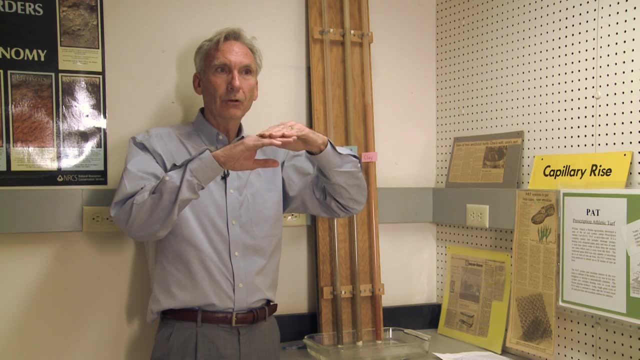 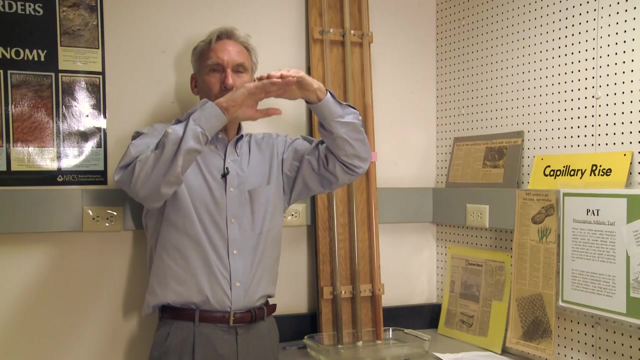 So why is this so important? So capillary rise in a soil and you have the water table, depending on what type of soil you have. if you have a very clay-textured soil, chances are it's going to migrate up. But what's going to happen is that the soil will migrate up and you're going to have 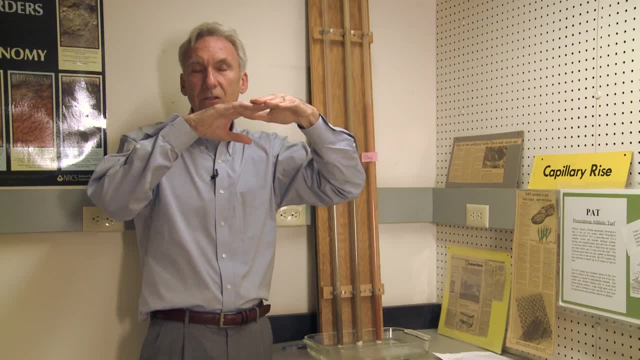 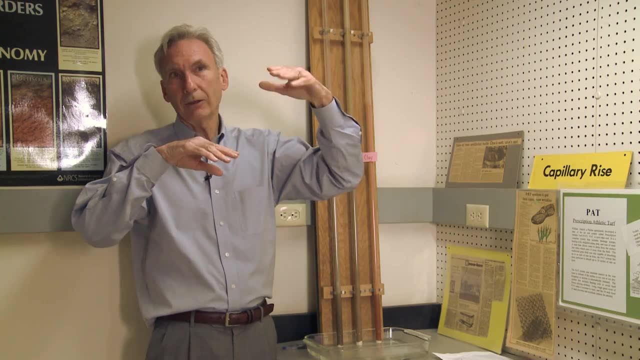 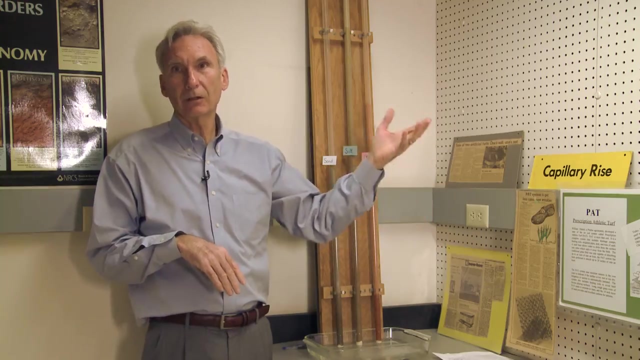 lots of water ponding all over the place. whereas with the sand you'd get water moving through quickly and it wouldn't migrate up very far. But with the silt it can move up the water table quite easily because of capillary rise.